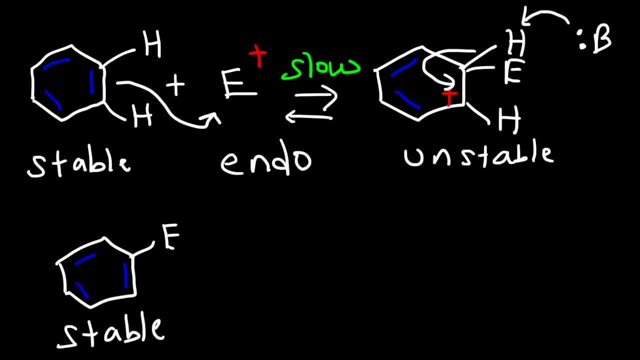 compound, And so the net result is that we replaced a hydrogen atom with an electrophile, So this is called an electrophilic aromatic substitution reaction. By the way, the second step for this process is fast, because we're going from an unstable compound to a stable compound, and also that step is 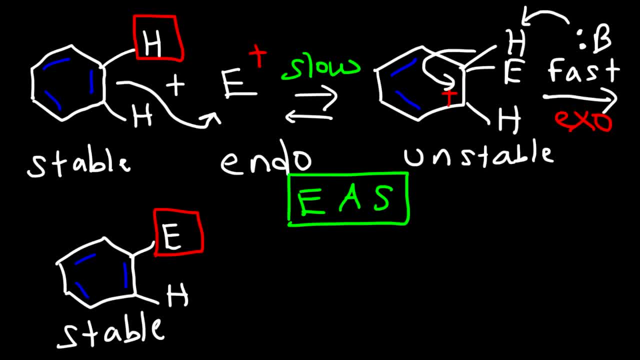 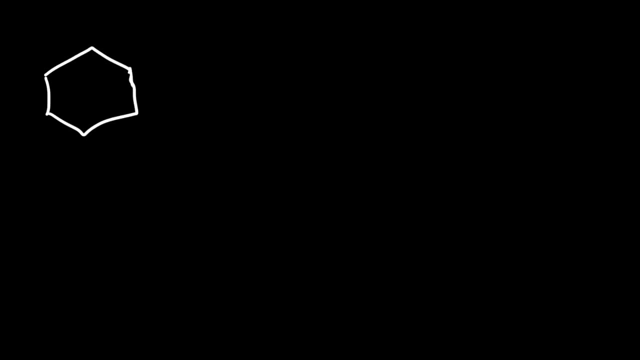 exothermic Energy is going to be released because we're going from a high-energy compound to a low-energy compound. So those are some things to keep in mind. And now let's go over the bromination of benzene. So here we have a benzene ring and we're going to react it with Br2 and with a Lewis acid. 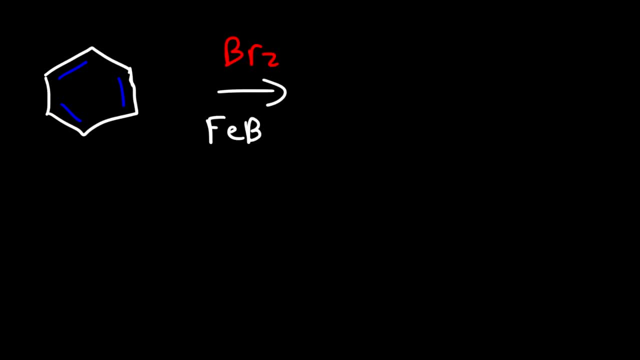 catalyst called FeBr3, iron bromide, And so we're going to replace the hydrogen atom with an electrophile. In this case, the electrophile is the bromine atom, And so that's how we can convert benzene into bromo-benzene. 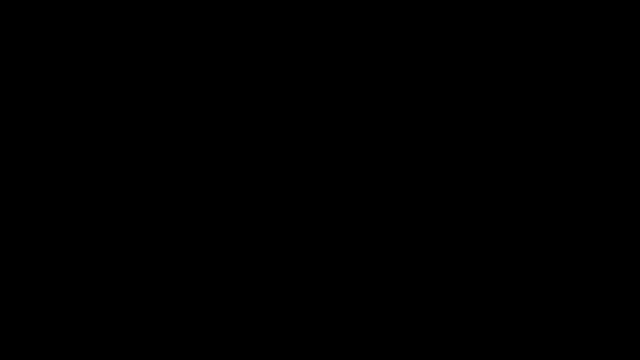 So let's write a mechanism for this reaction. So in the first step, bromine is going to react with the Lewis acid catalyst. Right now, each bromine atom has three lone pairs. Okay, And so bromine adds itself to FeBr3 in a reversible reaction and we're going to get this compound. 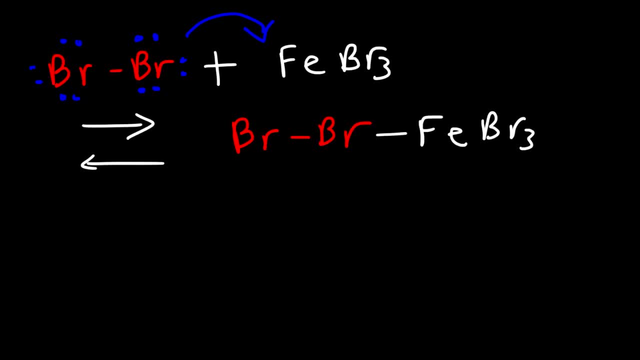 Whenever the Fe atom or the iron atom has four bonds, it's going to have a negative formal charge, And bromine, which now has two bonds, has a positive formal charge. So this is the species that we're going to react the benzene ring with. 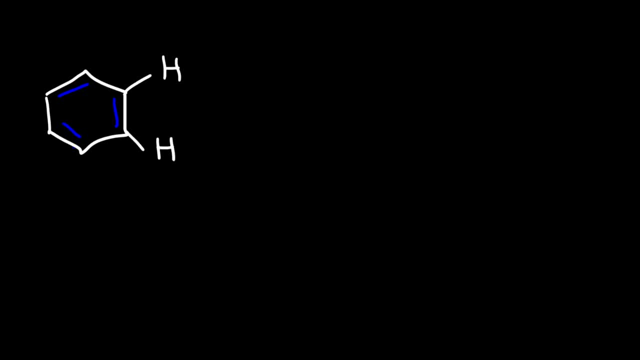 So, like always in an EAS reaction, that is, in an electrophilic aromatic substitution reaction, the benzene ring is going to behave as the nucleophile And a bromine atom at the far left is going to behave as the electrophile. 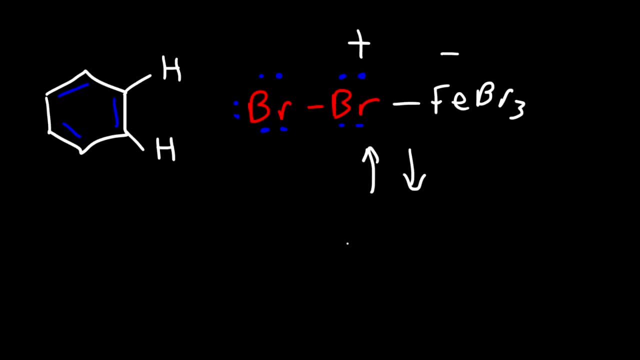 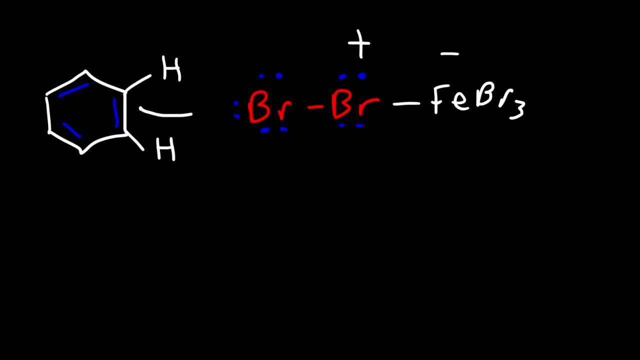 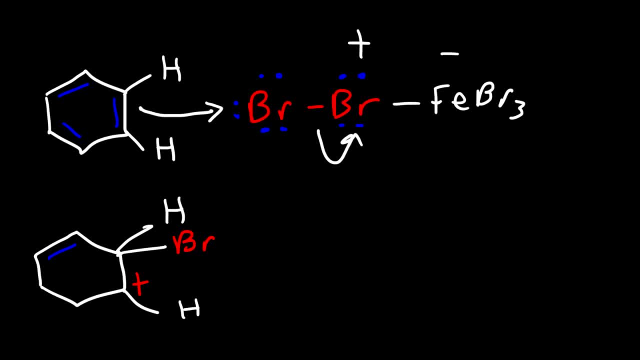 carbon. So between these two carbons, if you add a bromine atom to the top carbon, the positive charge will be at the bottom carbon, So it has to be on the other carbon that you add the bromine atom to Now. the next step is to use the base. In this case we 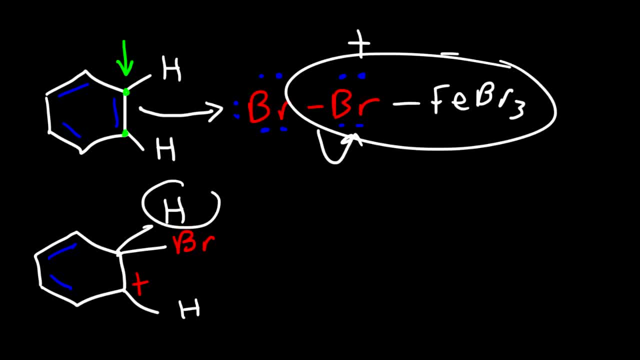 can use the solvent or this molecule to abstract a proton. So I'm going to use this molecule. So we have a bromine atom attached to FeBr3. And so FeBr4- which is this whole thing combined. it's going to act as a base and 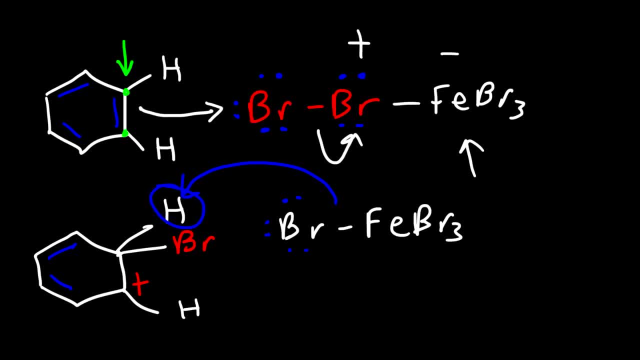 abstract the proton. This hydrogen is highly acidic because this compound is unstable, and so this sigma complex, or arenium ion as some textbooks call it, really wants to dish out this proton, because once it gets rid of it it can regenerate the aromatic ring, And so even a bromide ion will suffice as a base to get rid of that proton. 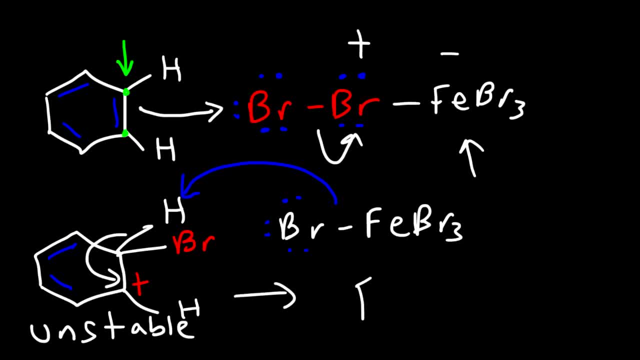 So once it's gone, we're going to have the aromatic ring. So once again we have a stable compound and this is going to be the final product. So that's the mechanism for the bromination of benzene. So the net effect is that we are replacing a hydrogen atom with an 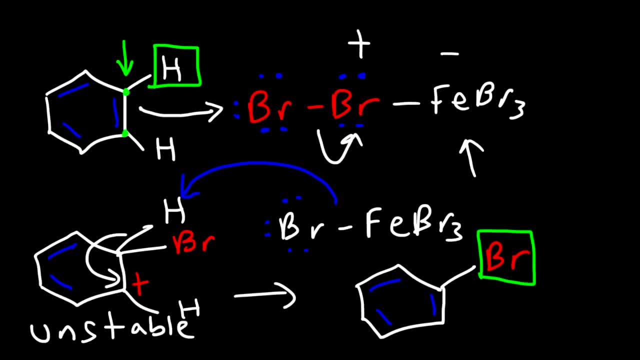 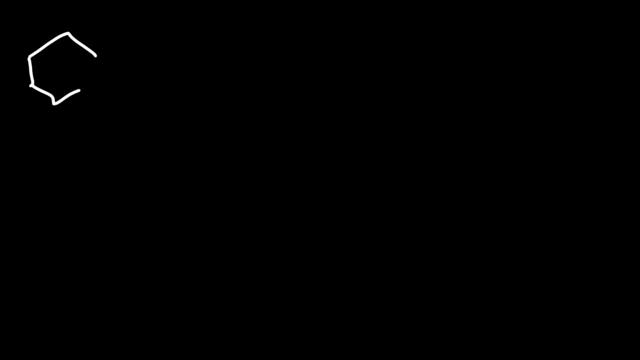 electrophile, a bromine atom, And so it's called an electrophilic aromatic atom Substitution reaction. Now let's move on to our next example, and that is the chlorination of benzene. So if we react benzene with chlorine gas and AlCl3, 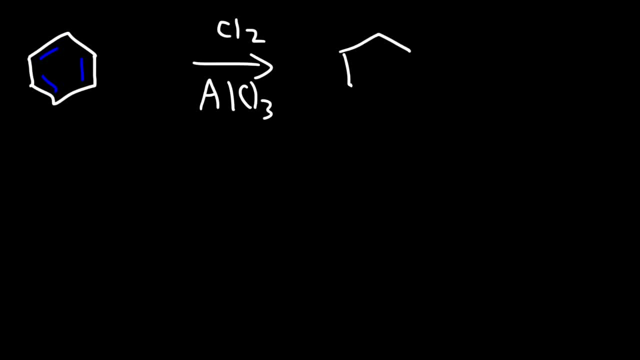 aluminum chloride. this will generate chlorobenzene, which looks like this. By the way, in addition to using AlCl3, you could also use FeCl3. So both of these Lewis acid catalysts can work in this reaction, But for this. 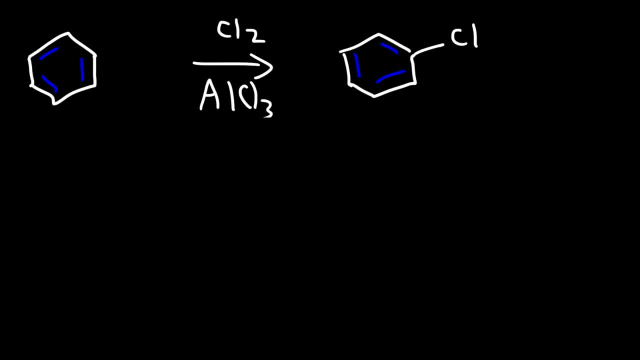 example, I'm going to use AlCl3.. So in this mechanism, which is similar to the last one, the chlorine atom- I mean the chlorine molecule rather- will react with the Lewis acid catalyst. So basically, it's going to add itself to that catalyst. 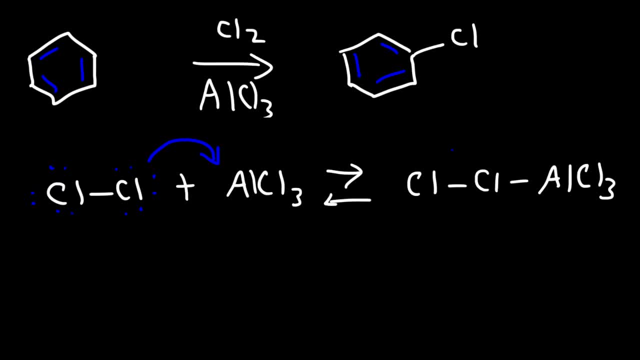 Given us this intermediate, where the aluminum atom has a negative charge, that is, a negative formal charge, and the chlorine atom attached to it has a positive formal charge, And so the benzene ring is going to attack this species, just like it did before. 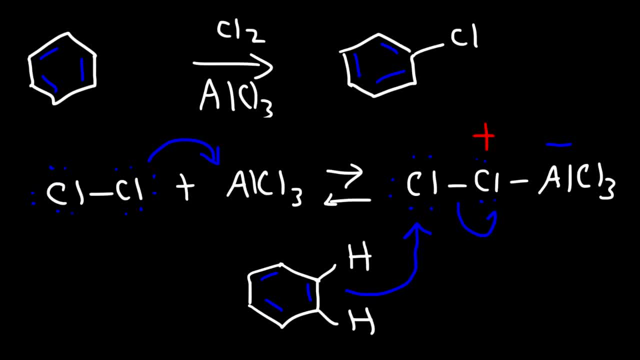 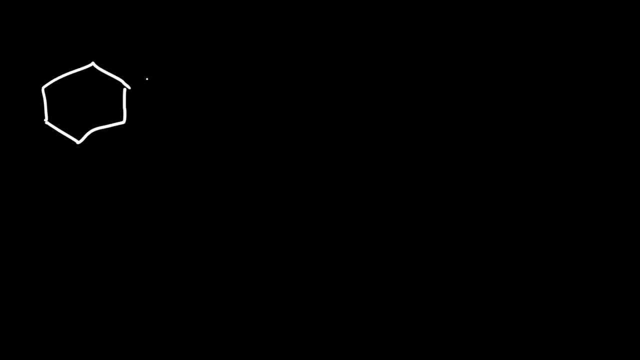 So it's going to attack this chlorine atom and expel in this group. So here is the chlorine atom and we're going to get a sigma complex, which is basically a carbocation inside of what used to be a benzene ring, And then in. 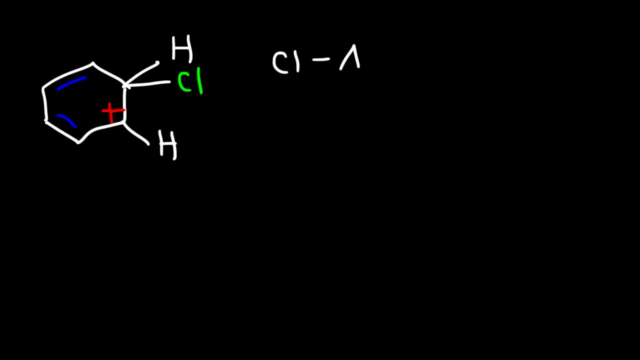 the next step. the base is going to come in, which is AlCl4. And it's going to grab a hydrogen regenerating the benzene ring. So we're going to get chlorobenzene as our product, And then we're also going to get HTL. 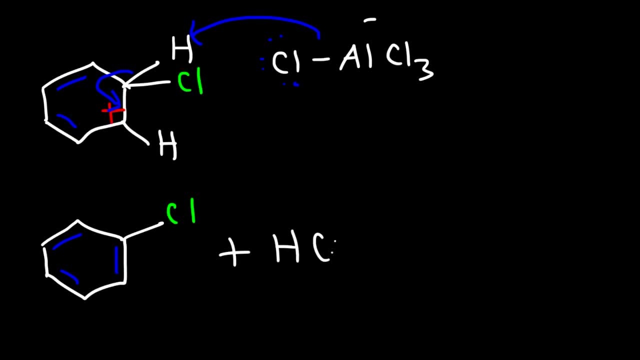 As another side product, And we're also going to regenerate the aluminum chloride catalyst. So because AlCl3 was regenerated in a reaction, it wasn't consumed in a reaction. It is therefore a catalyst. Now we're going to go over one last reaction, and that is the iodination of benzene. 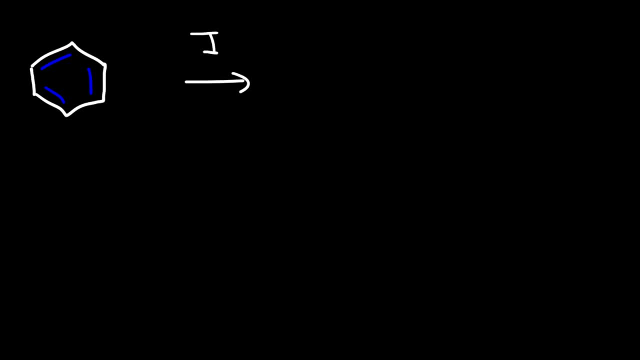 So if we react benzene with iodine using an oxidizing agent under acidic conditions like nitric acid, we can get iodobenzene. Now there are some other reagents that we could use as well, For example, another one that can accomplish: 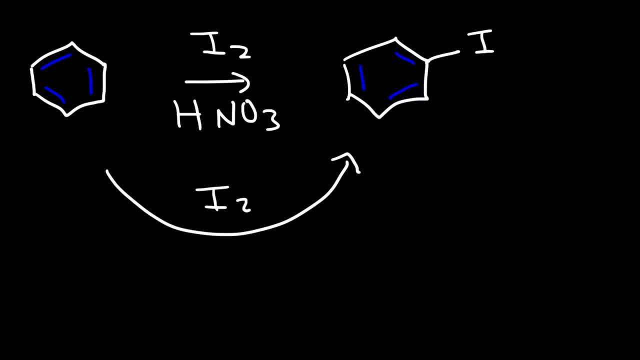 this transformation is using iodine with hydrogen peroxide and sulfuric acid. I've also seen iodine with hydrogen peroxide and sulfuric acid. I've also seen iodine with hydrogen peroxide and sulfuric acid. I've also seen that example too. So that's how you can convert benzene into iodobenzene, And so 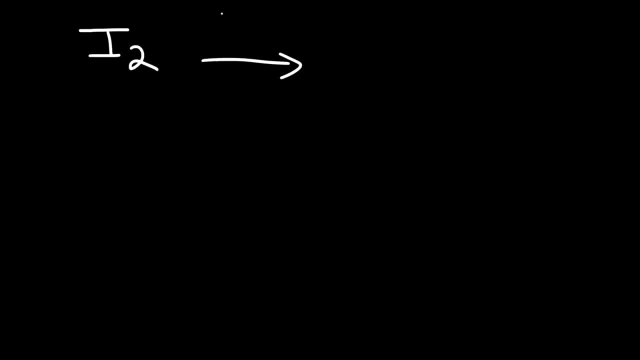 what happens is that the oxidizing agent oxidizes iodine from its neutral state to a positive one oxidation state, And so that is the electrophile that reacts with the benzene ring, And here is the general mechanism for it, which is very similar. 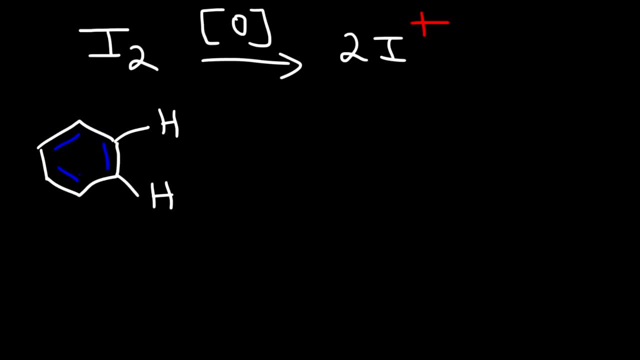 to the other mechanisms that we've been doing. So the benzene ring is going to behave as a nucleophile and it's going to react with this electrophile, And so I'm going to add the iodine atom to the same position. I'm going to follow the same process, which. 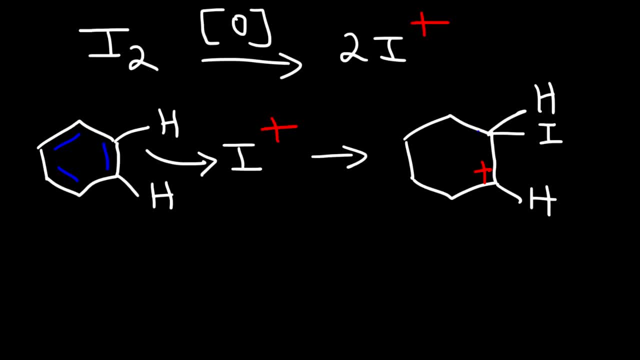 means we're going to have a positive charge on this carbon. So that's our carbocation intermediate, And then some base in the solution- it could be the solvent, or it could be something else- is going to basically take away that proton, And so we're going to. 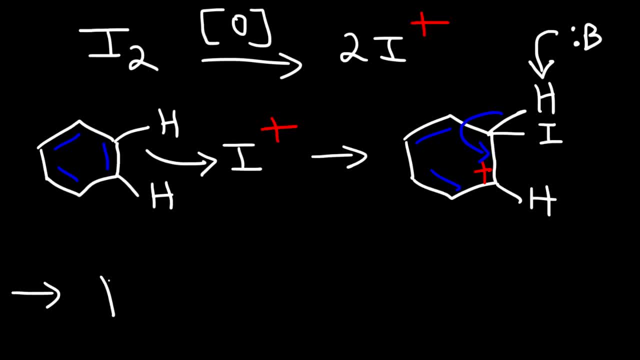 regenerate the aromatic ring, thus given us iodobenzene, which looks like this, And so that's it for this video. So now you basically have the generic mechanism for the halogenation of an aromatic ring such as benzene. So thanks for watching.